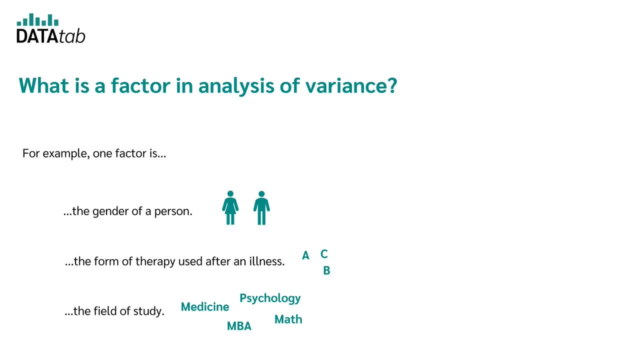 of analysis of variance. a factor is therefore a categorical variable. You use an analysis of variance whenever you want to test whether these categories have an influence on the so-called dependent variable. For example, you could test whether gender has an influence on salary, whether the therapy has an influence on the blood pressure or whether 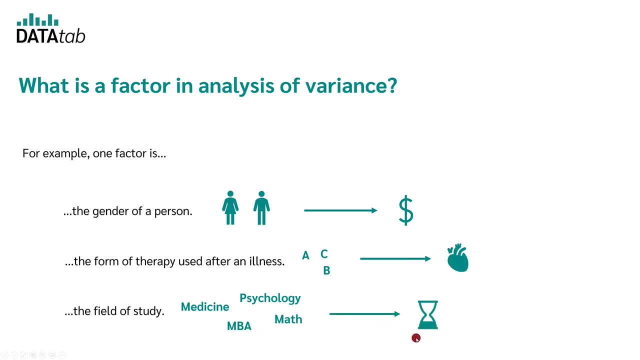 the field of study has an influence on the duration of study. Salary, blood pressure and study duration are then the dependent variables. In all these cases, you can now check whether the factor has an influence on the dependent variable. Since you only have one factor, in these cases you could use a single-factor. 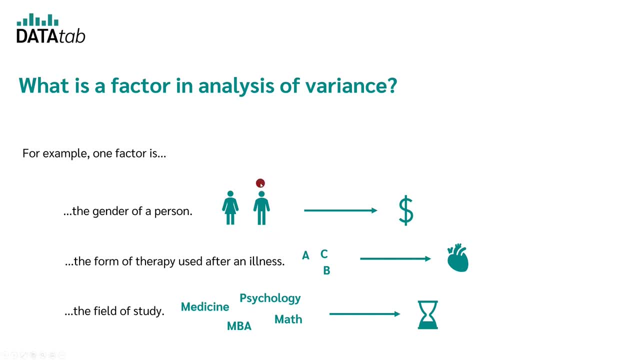 analysis of variance. You're right if you say: well, in the first case we have a variable with only two categories, so of course we could use the t-test for independent samples as well. Now, of course you may say: but I have another categorical variable that may also have an effect on the 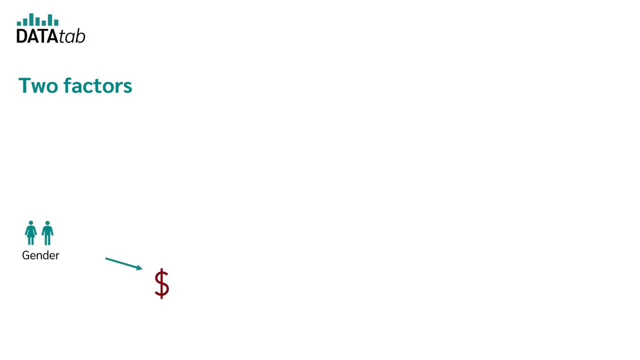 dependent variable, and I want to include that variable as well. Maybe you would also like to know if, in addition to gender, the highest level of education has an impact on salary, Or in addition to the form of therapy. maybe you would also like to include gender Or in your 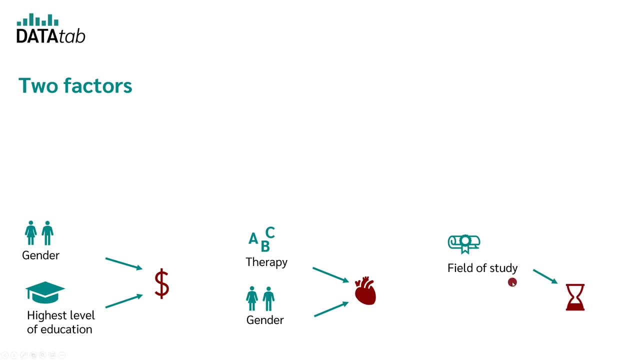 third case, you would also like to know whether, in addition to the field of study, the university attended also has an influence on the length of study. Now, in these cases, you would not have one factor, but two factors in each case, And since you now have two factors, you use the two-factor. 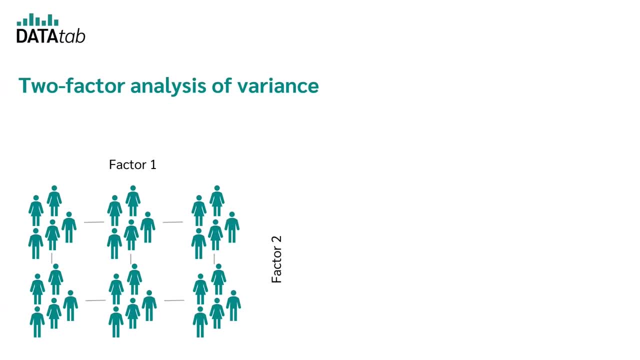 analysis of variance. With the help of the two-factor analysis of variance, you can now answer three things: Once whether the first factor has an influence on the dependent variable, Once whether the second factor has an influence on a dependent variable, And then you can also make a statement whether there is a so-called interaction effect between.